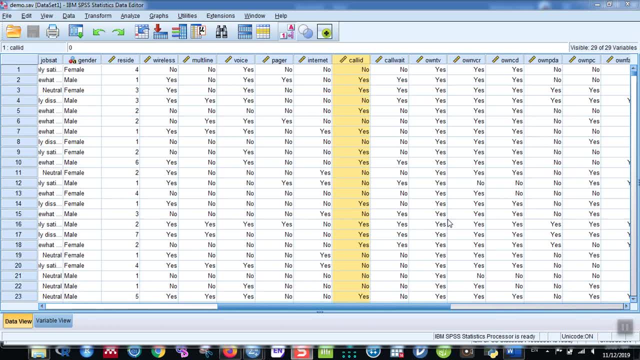 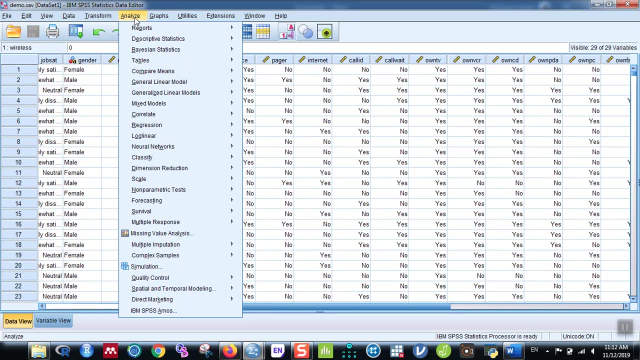 hello everyone, welcome back to my channel. this is Raz, So in this video I'm going to explain how to perform the multiple response analysis using SPSS. So let me go to the steps directly. okay, so go to analyze. okay, go to analyze and then go to multiple response and click on define variable sets. okay, so on the 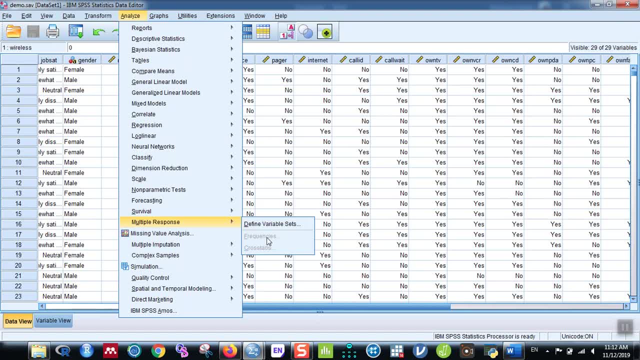 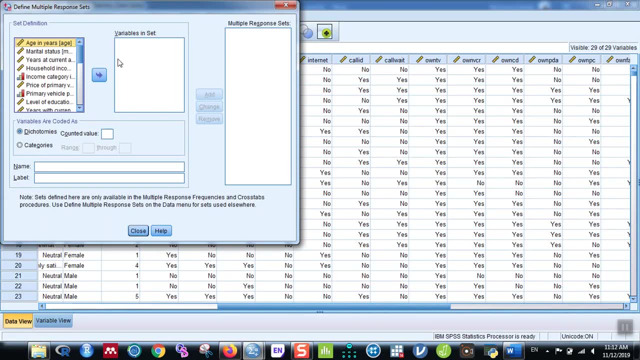 bottom of that you can see frequencies and cross tabs, but they are not highlighted. it cannot click on those because we have not defined the variable sets. so click on that. here you can see variables in set. okay, so what it means is that you have to put all those variables which are a part of multiple 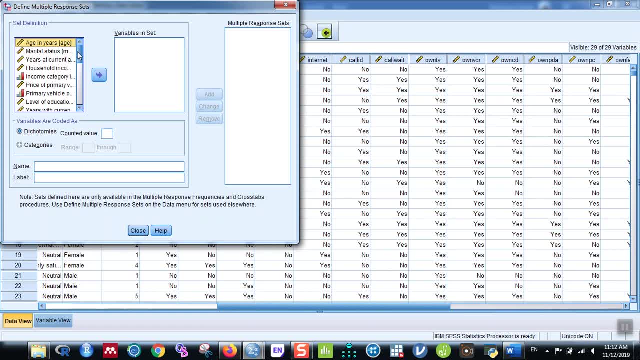 response. for example, you want to know what percentage of the people are using which means of communication- and there is a question in this data set, and what is the means of communication that you have at our house? or then there are several answers. so, for example, the people might have: 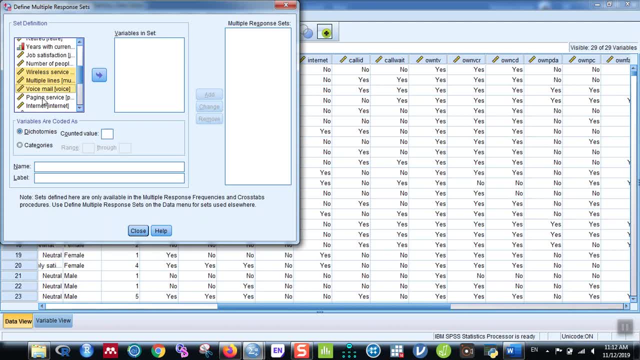 wireless services. they might have multiple lines: voicemail paging services, internet caller ID call waiting, television VCR studio, for example. these are the different options. okay, and then you can see. variables are coded as categories and dichotomies. okay, so here they are coded as the yes and no, and then you have to be: 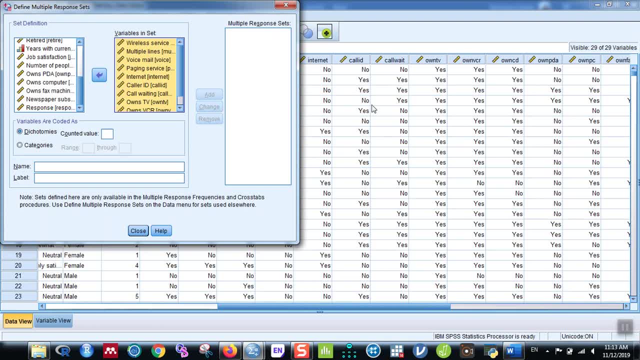 careful in identifying which codes are used for yes and which codes are used for but no. so in this data set one means yes and no is represented by zero. so here in countered value I put one okay, because one means yes in this data set, and then I have to keep the name and label. 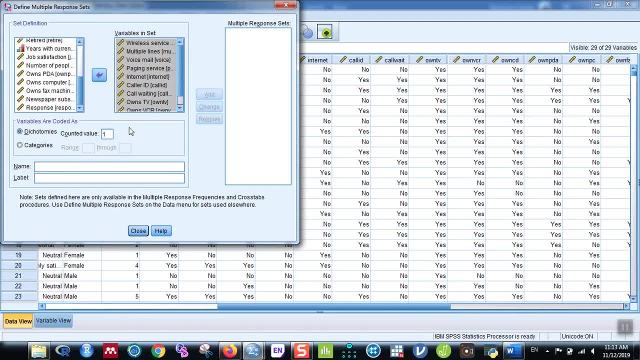 so these all are the part of the means of communication. so i can give a variable name: means means communication and in the label, means of communication, household. okay, and click on add. you can see that the multiple response set- one set, is created here so you can create many more sets depending on your questionnaire. so in